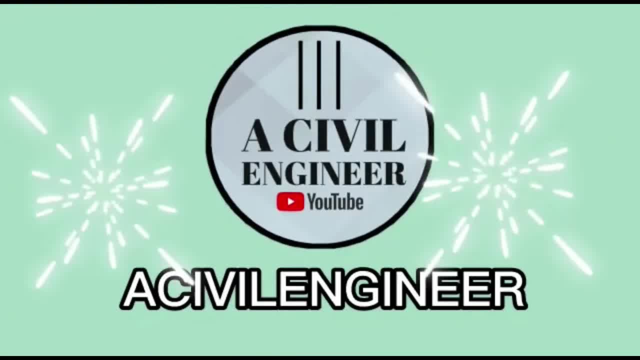 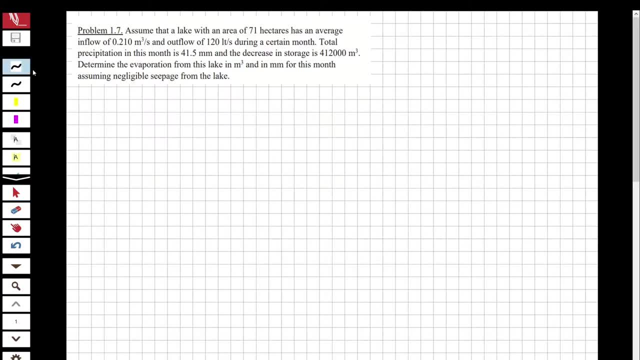 Hi guys, welcome to my channel. In this video we are going to solve the questions about engineering hydrology, and the question will be determining the evaporation of the lake. So let's solve the question. First we are going to read it: Assume that a lake with an 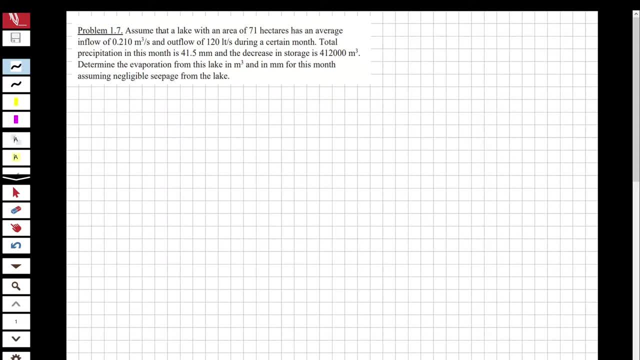 area of 71 hectares has an average inflow of 0.21 m3 per second and outflow of 120 liter per second during a certain month. Total precipitation in this month is 41.5 and the decrease in storage is 412,000 m3.. Determine the evaporation from this lake in m3 and mm. 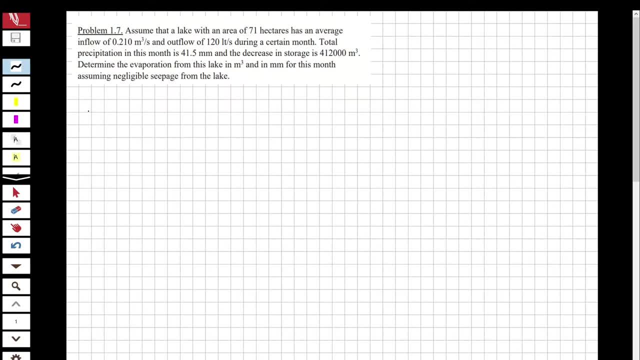 for this month, assuming negligible seepage from the lake. So we are going to seepage will be neglect. Okay, we are going to seepage, We are going to neglect the seepage. Let's calculate what is inflow and what we have. 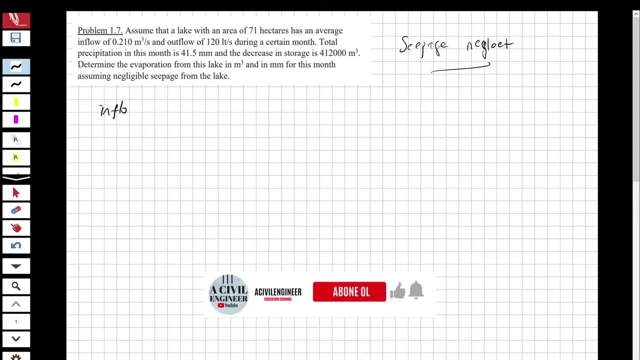 as outflow. For inflow now we have 0.21 m3 per second. Okay, so we have to convert it to the m3.. So we are going to multiply. I'm going to show you by the units: m3 per second. 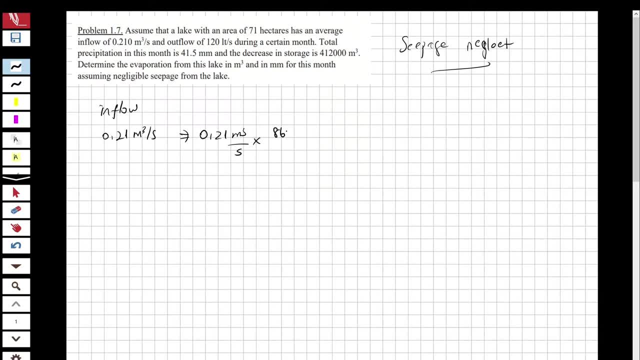 raise from 1, and we are going to multiply. We are going to read 86400 second over one day and multiply it in thirds. sorry, multiply it 30 days over one month, and this we are going to obtain the maximum rate of over one month in case the bear volcano will break. 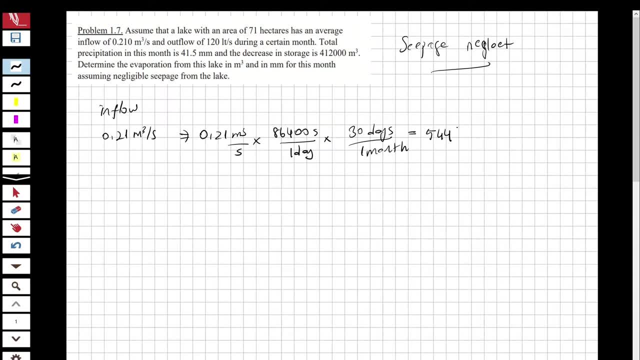 five hundred forty four thousand three hundred twenty meter cubic as the inflow water. the water comes to the our lake. okay, so we have an also outflow that we lost the water it gets out from the lake. so what is outflow? outflow is 120 liter. yeah, liter liter per second. so for this one we are 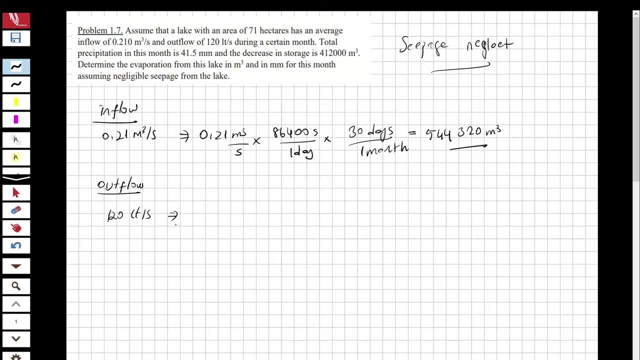 going to convert it to meter cubic. if you want to convert to meter cubic, we are going to divide 120 or 1,000. 120 over 1,000, we are going to obtain, or point, 12 meter cubic per second. and now we are. 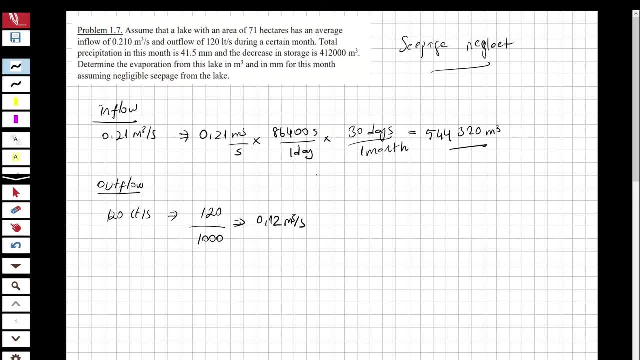 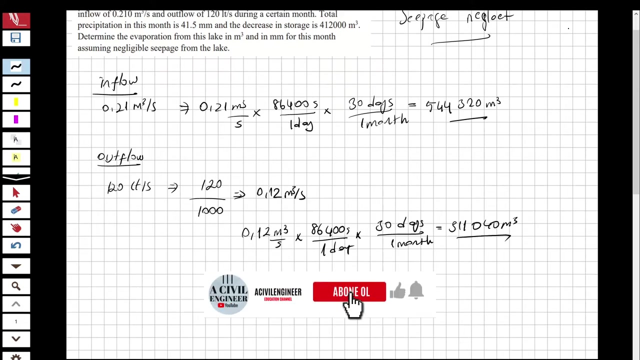 going to write also for the outflow, the same multiplication of 0.12. I'm gonna write here: 0.12 meter cubic per second, multiplied 86 400 second over one day, and multiply 30 days for one month, and we are going to obtain 311 040 meter cubic. now this is also outflow. so let's calculate the. 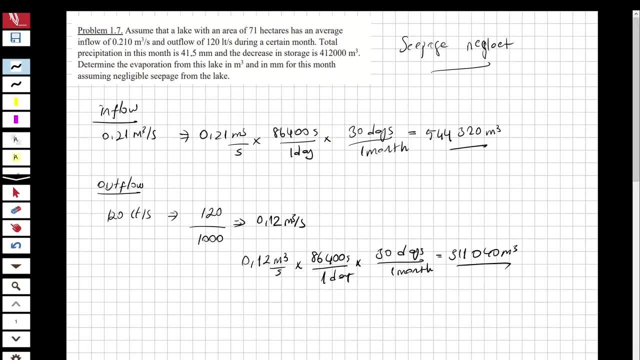 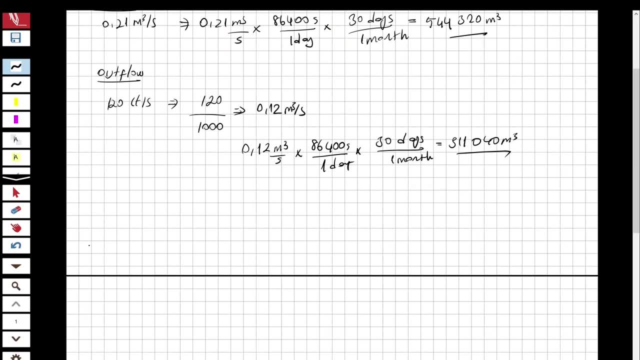 precipitation, because you can see here 41.5 millimeter as a precipitation for the month. let's find it. this is precipitation, okay, and 41.5 millimeter we are going to convert to a meter, so i'm going to divide this thousand and this will be equal to 0.0415 as meter. okay, now we have the in terms of meters, so let's calculate. 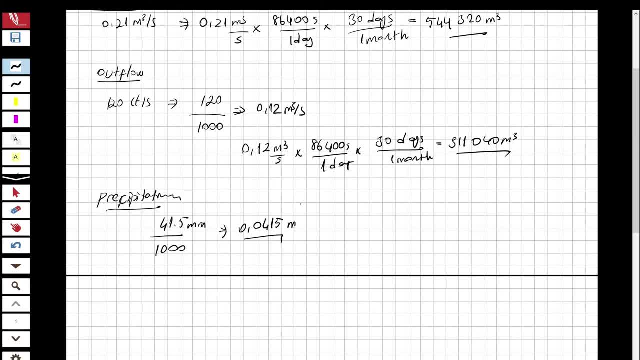 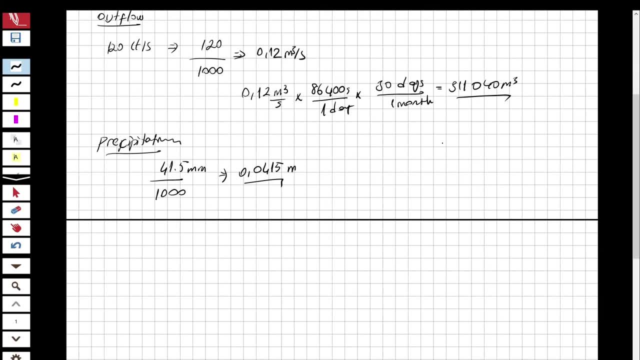 it. let's find the total volume of that, the total volume respect to this area. what is the area? 71 hectare, right? so this is going to be 0.0415 multiplied 71 and multiplied 10 000, because one hectare is equal to 10 000 meter square. 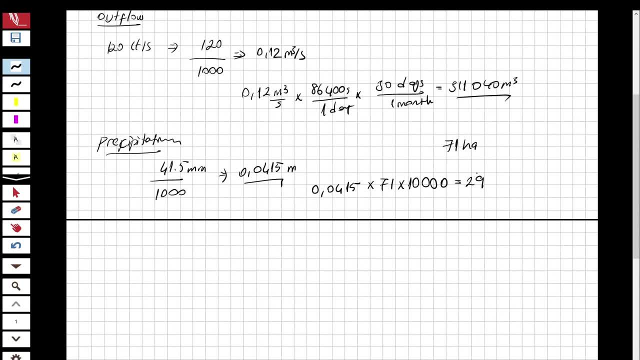 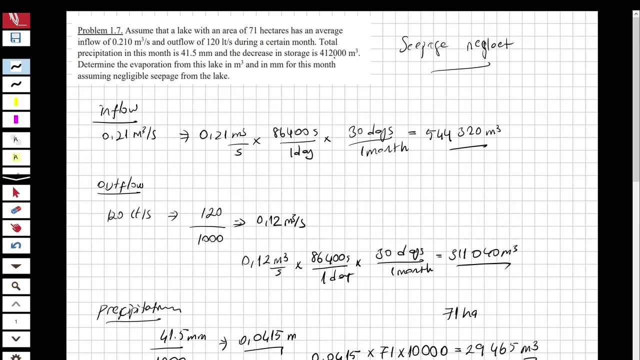 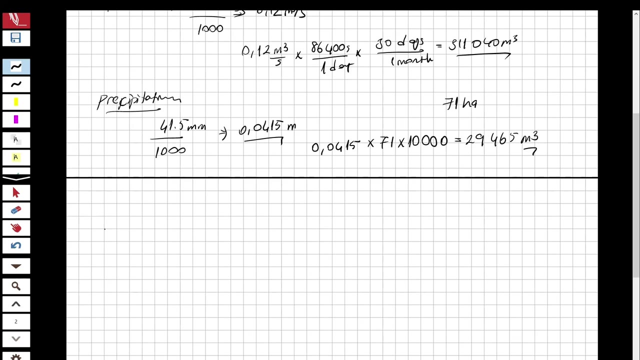 and this will be equal to 29 465 meter cubic. now we determine these all and also we have a decrease in the storage. look at here decreasing storage of storage: four thousand twelve, yeah, four, sorry, four hundred, uh, twelve thousand meter cubic. so let's write this. we are going to write the, the positive ones and the.